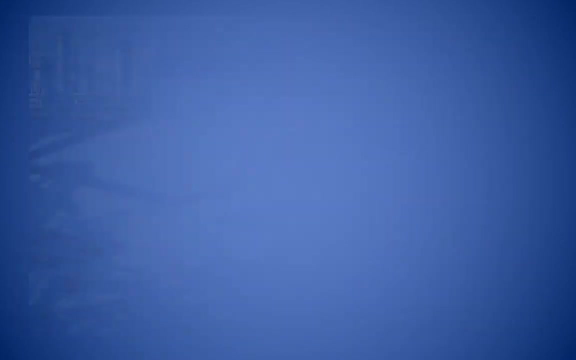 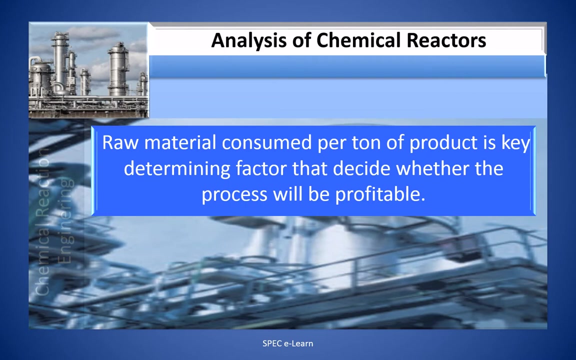 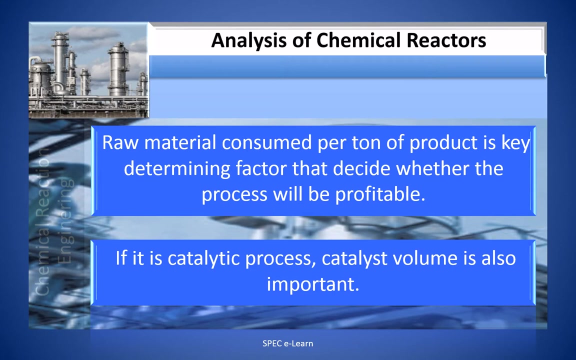 This reactor is a hot of the plant. It is a reactor performance that makes a process economical or not. Contact with iy, the reactor coin Reactor material. Consumed pattern of product is a key determining factor that decide whether the process will be profitable. 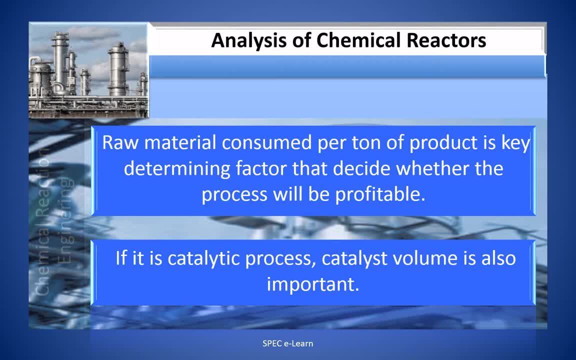 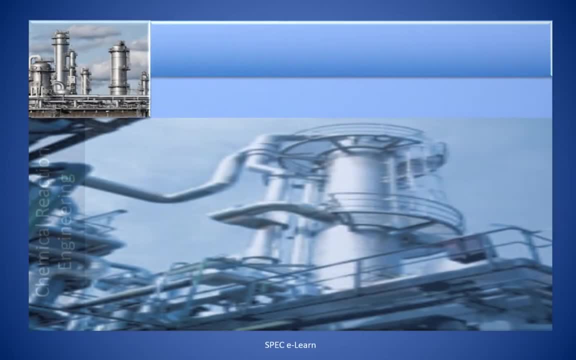 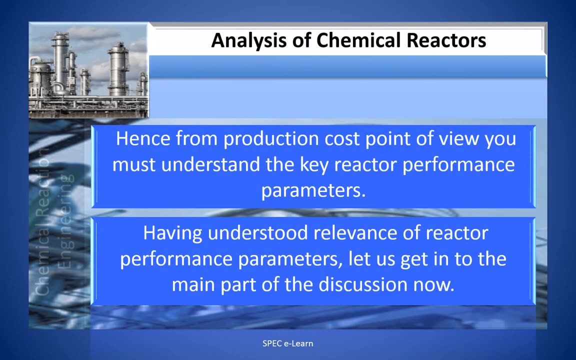 If it is a catalytic process, catalyst volume is also important. Hence, from production cost point of view, you must understand the key reactor performance parameters. Having understood the relevance of reactor performance parameter, let us get into the main part of the discussion now. 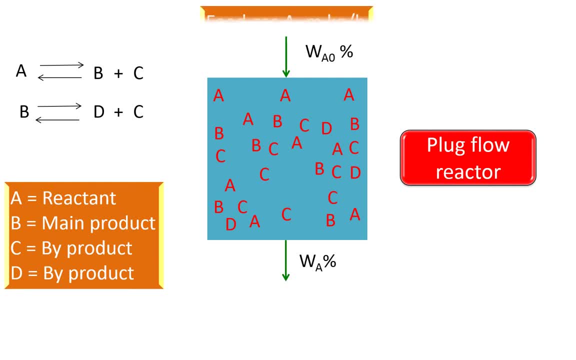 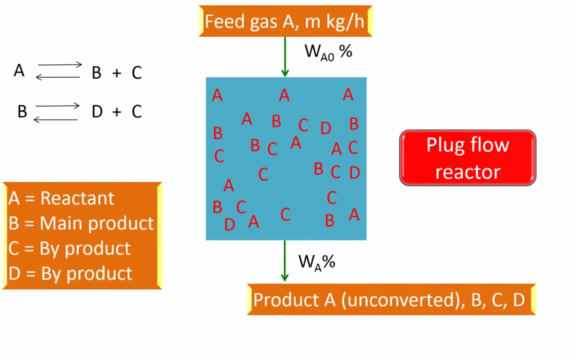 Shown in this figure is a plug flow reactor. Reactant A reacts to form product B and C, the first reaction. The product B that forms the first reaction, further reacts to form D. So the reactor output contains unreacted A products B, C and D. 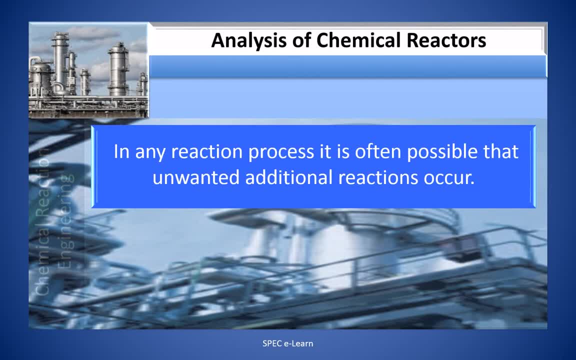 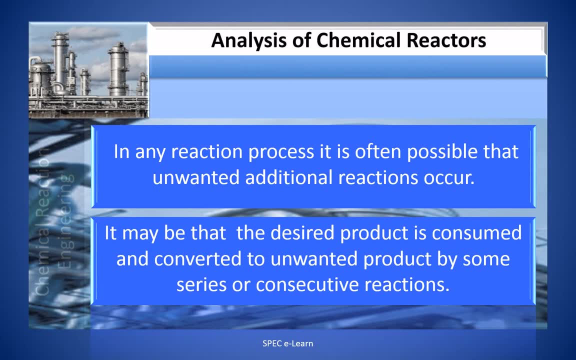 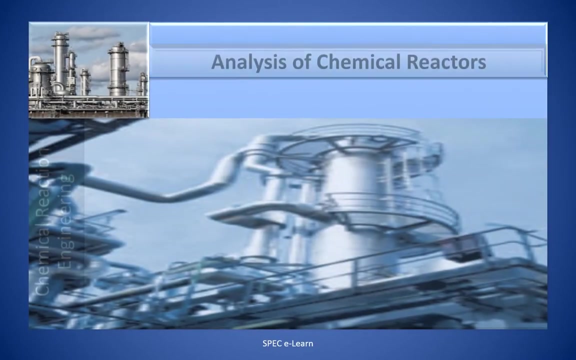 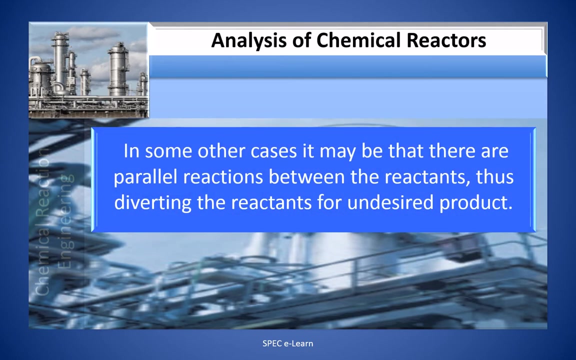 In any reaction process it is often possible that unwanted additional reaction occur. It may be that the desired product is consumed and converted to unwanted product by some series or consecutive reactions. In some other cases it may be that there are parallel reactions occurring between the 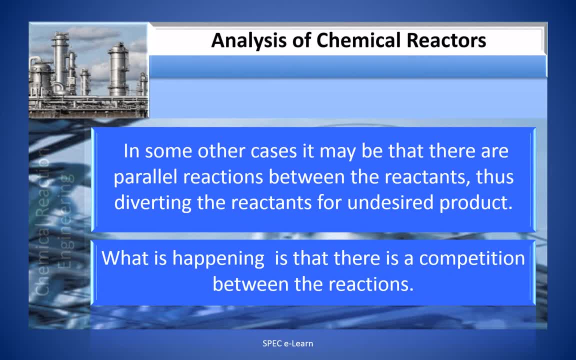 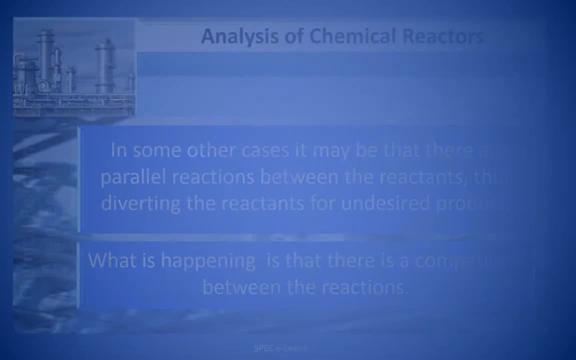 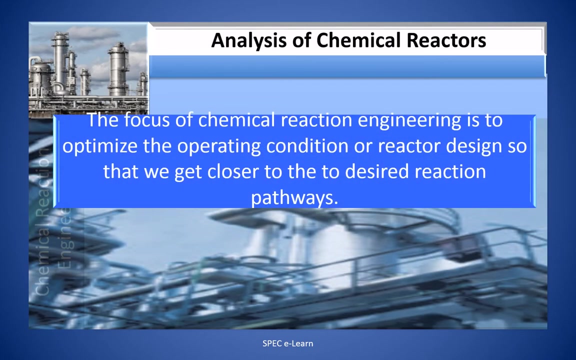 reactants, Thus diverting the reactants for undesired product. What is happening is that there is a competition between the reactions. The focus of chemical reaction engineering is to optimize the operating conditions or the design so that we get closer to the desired reaction pathways. 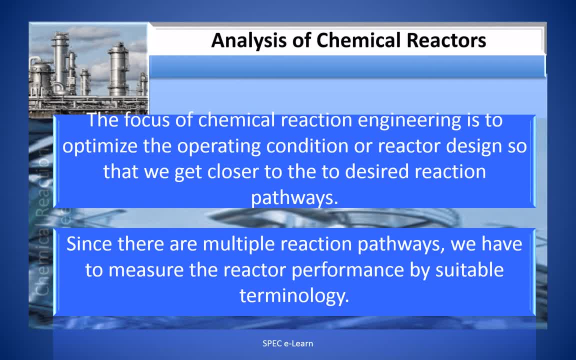 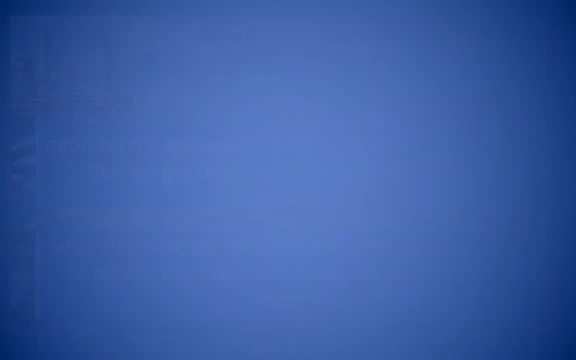 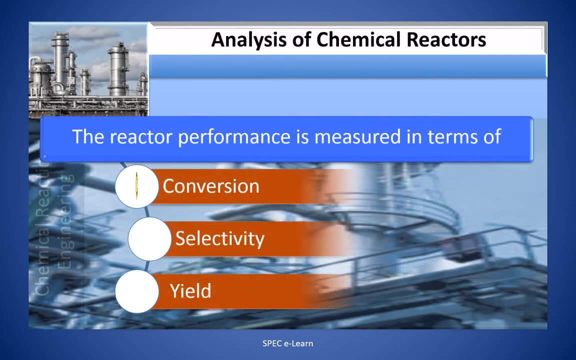 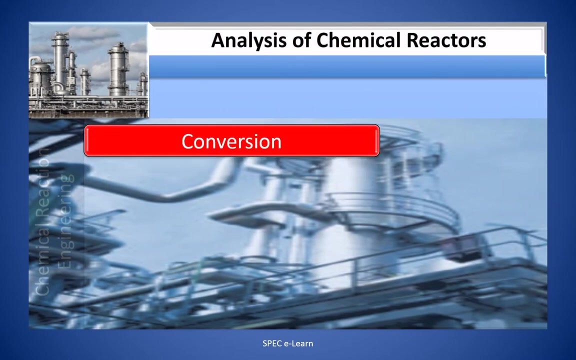 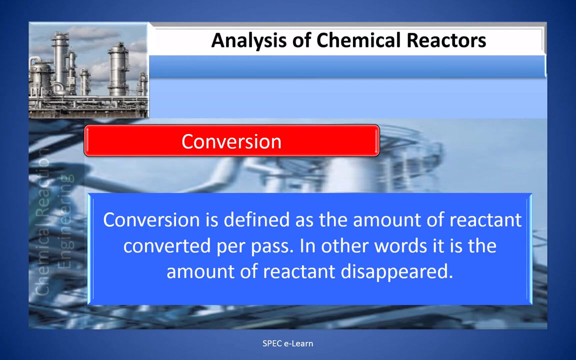 Since there are multiple reaction pathways, we have to measure the reactor performance by suitable terminology. The reactor performance is measured in terms of conversion, selectivity and efficiency. The reactor performance is measured in terms of conversion, selectivity and efficiency. Now let us move on to understand what these terms actually mean when applied to 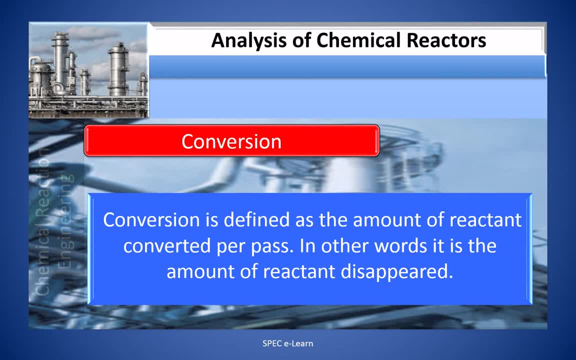 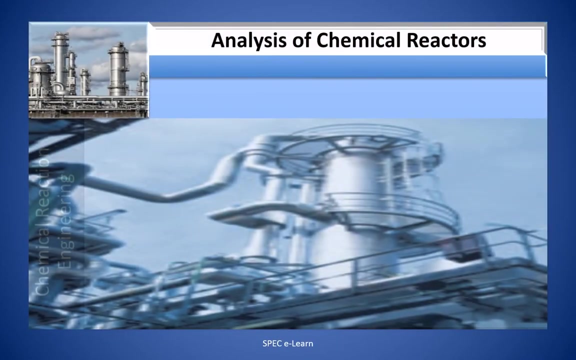 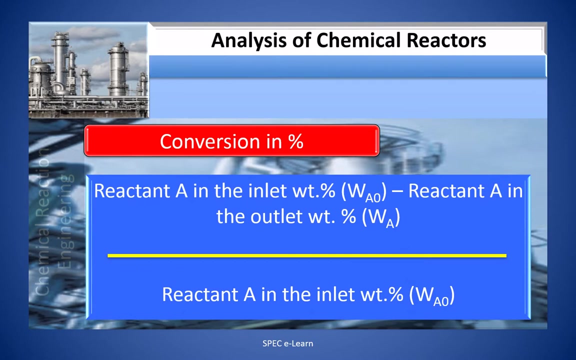 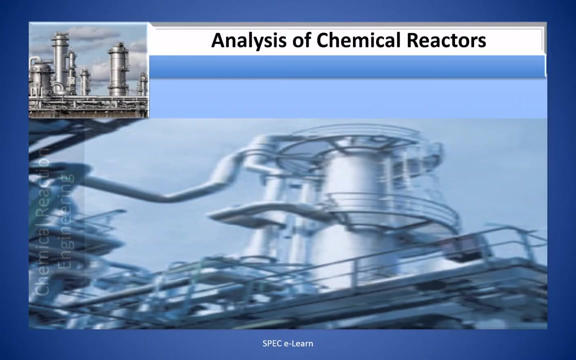 analyzing reactor performance. First, conversion Minus conversion. Conversion is defined as amount of reactant converted per pass. In other words it is amount of reactant disappeared. It is a ratio of reactant A in the inlet, in weight percent, minus reactant A in the outlet, in weight percent, to the reactant A in the inlet in weight percent. 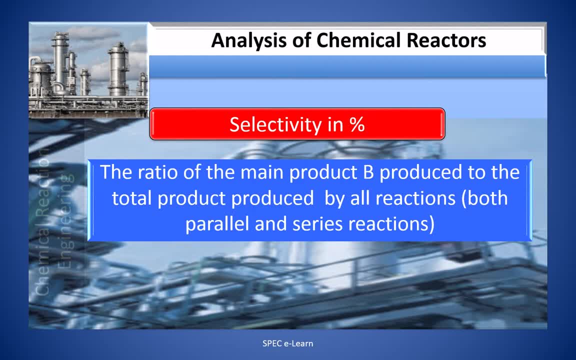 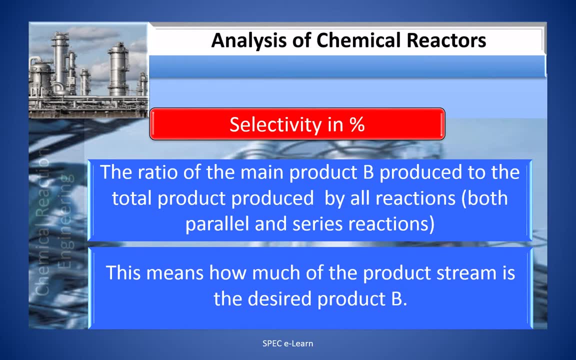 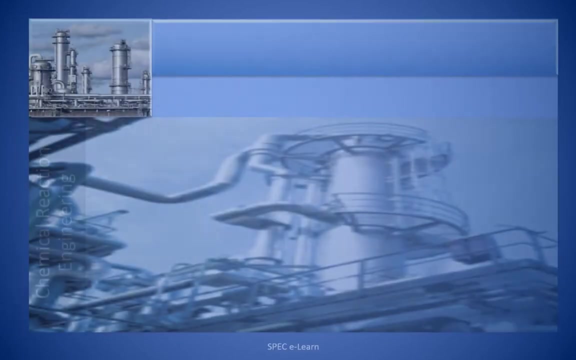 The second term applied to analyze reactor performance is selectivity. Selectivity is the number of reactants in the reactor. It is the ratio of the main product B produced to a total product produced by all reactions, both parallel and series reactions. This means how much of the product stream is a desired product B. 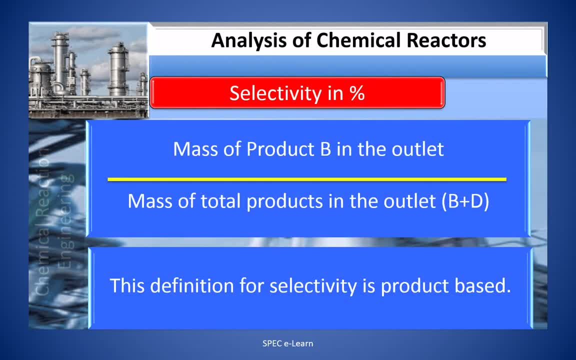 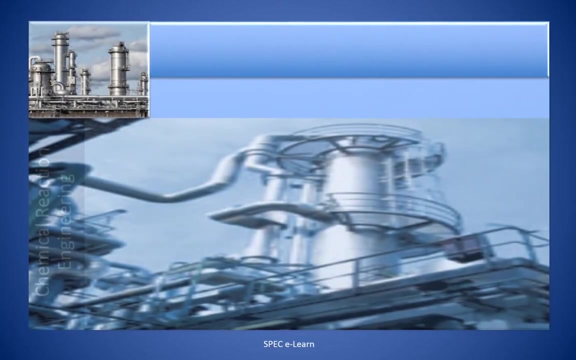 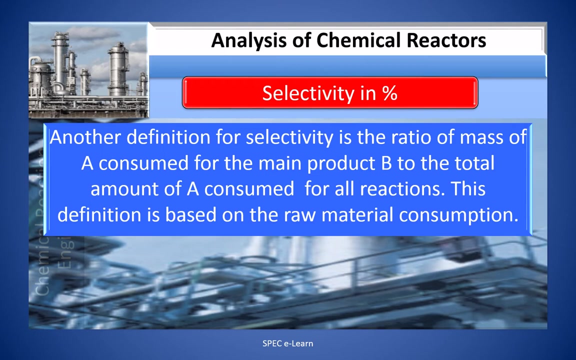 Expressing is an equation. Selectivity is the number of reactants in the reactor. It is the ratio of mass of product B in the outlet to the mass of total product in the outlet. This definition for selectivity is product-based. Another definition for selectivity is a ratio of mass of A consumed for the main product B to the mass of total product B. 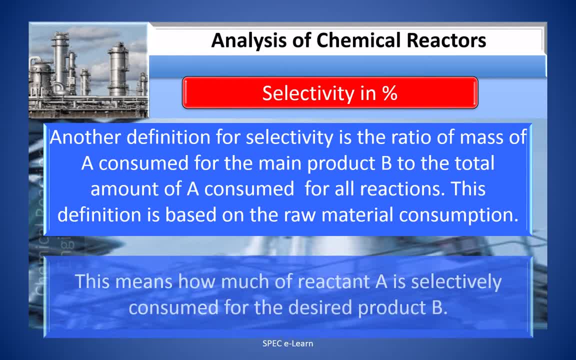 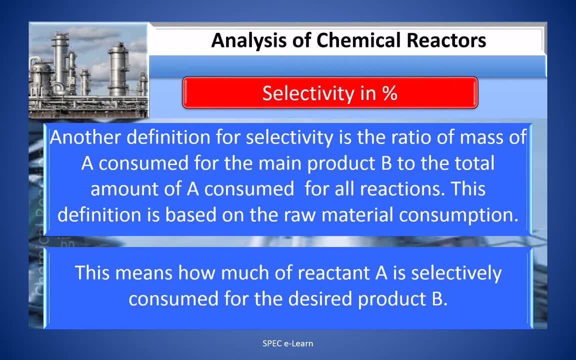 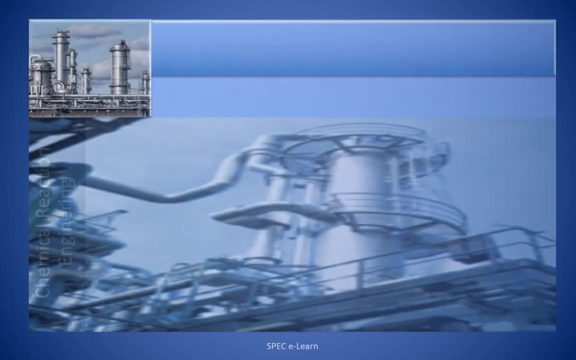 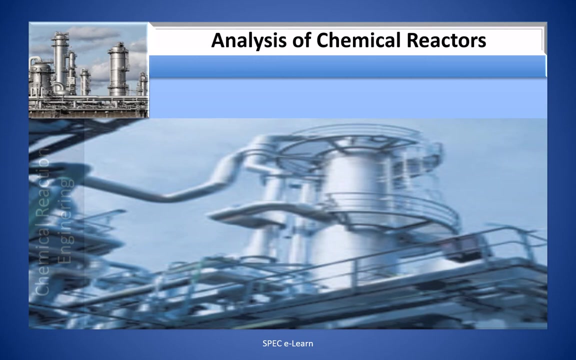 A consumed for the main product B to the total amount of A consumed for all reactions. This definition is based on the raw material consumption. This means how much of reactant A is selectively consumed for the desired product B. Selectivity based on products is generally used for analyzing reactor performance. 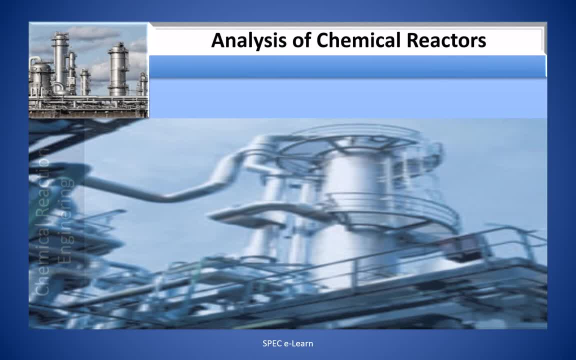 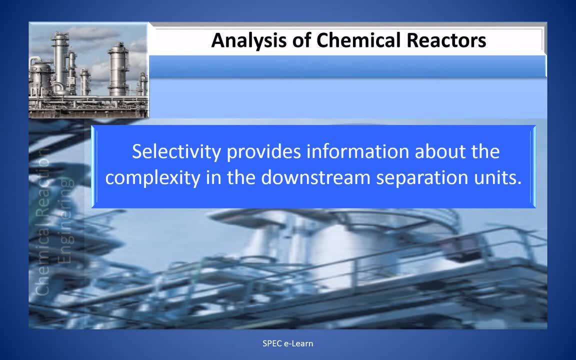 So do not confuse with the definition. It is only to understand the terminology in different context, which will help us to understand the process. better Selectivity provides information about the complexity in the downstream separation units. Lower selectivity means more by-products in the system. 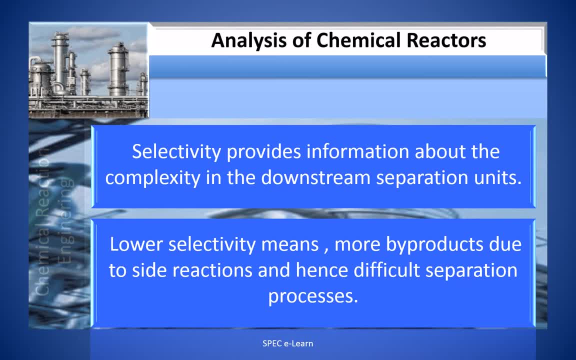 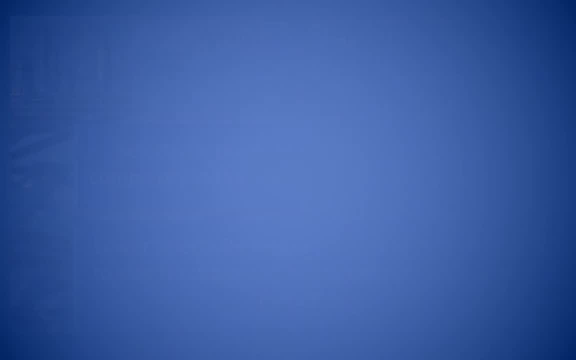 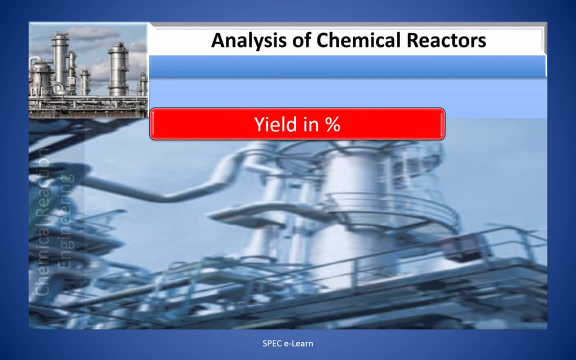 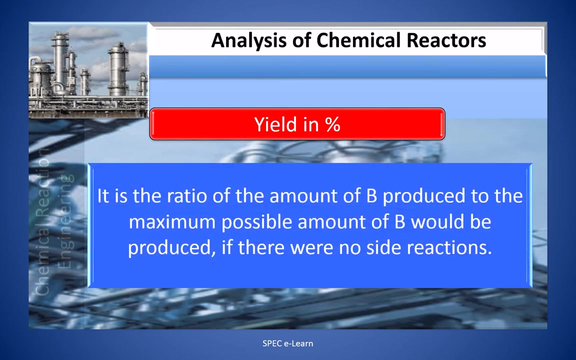 Over selectivity means more product B due to side reactions, hence difficult separation processes. The third important performance metric in analyzing reactor performance is yield. Yield is the ratio of the amount of product B produced to the maximum possible amount of product B would be produced if there were no side reactions. 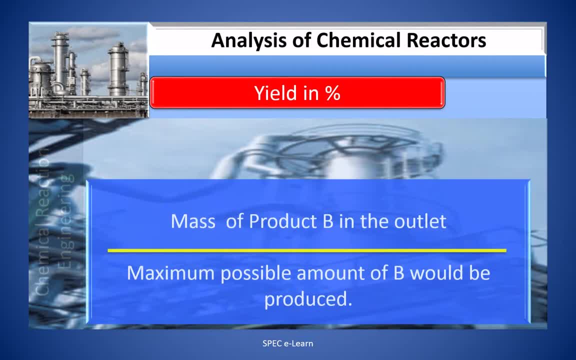 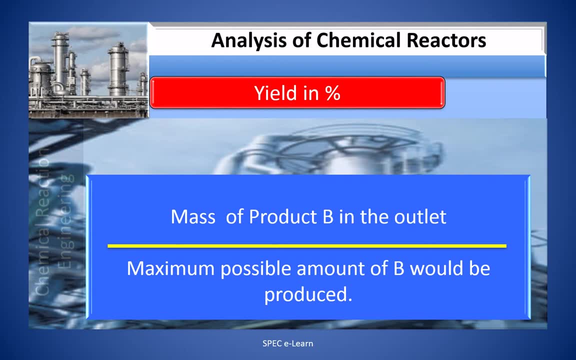 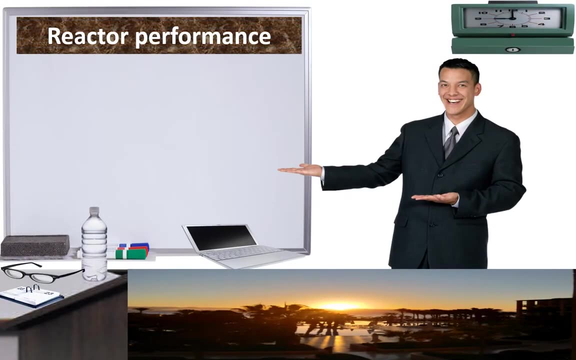 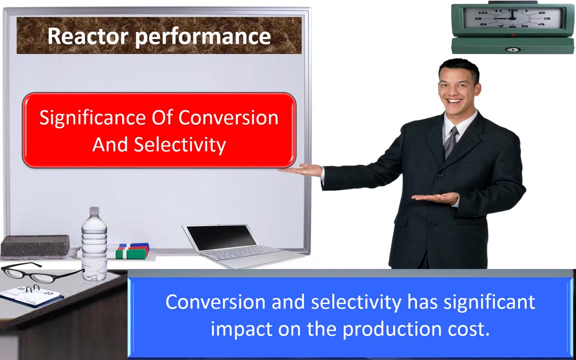 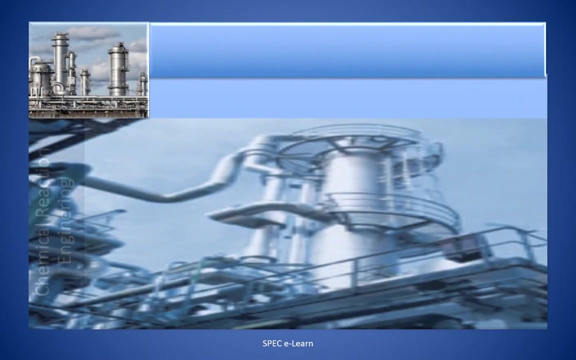 So yield is given by mass of product B in the outlet, divided by maximum possible amount of B would be produced if there were no side reactions. Significance of conversion and selectivity. Conversion and selectivity has a significant impact on the production cost. Higher conversion means lower recycle flow rate. 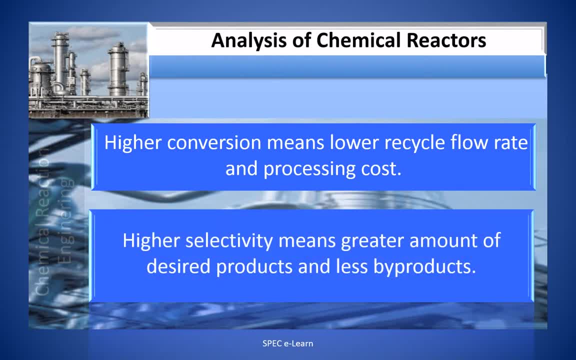 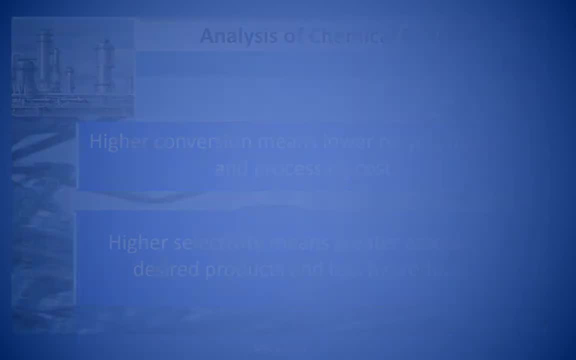 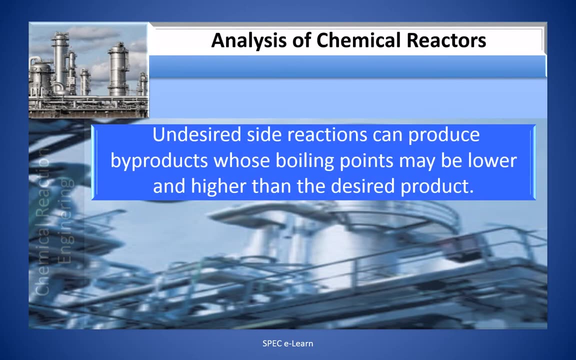 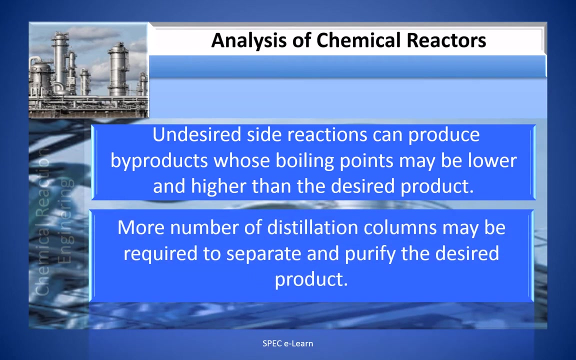 and processing cost. Higher selectivity means greater amount of desired products and less byproducts. Undesired side reactions can produce byproducts whose boiling points may be lower or higher than the desired product. More number of distillation columns may be required to separate and purify the desired product. 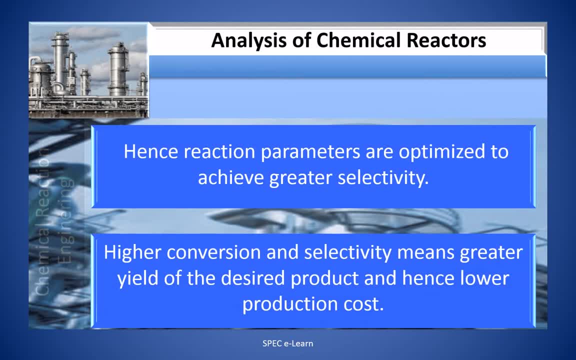 Hence reaction parameters are optimized to achieve greater selectivity. Higher conversion selectivity means greater yield of the desired product, hence lower production cost. More number of distillation columns may be required to separate and purify the desired product. Hence reaction parameters are optimized to achieve greater selectivity. 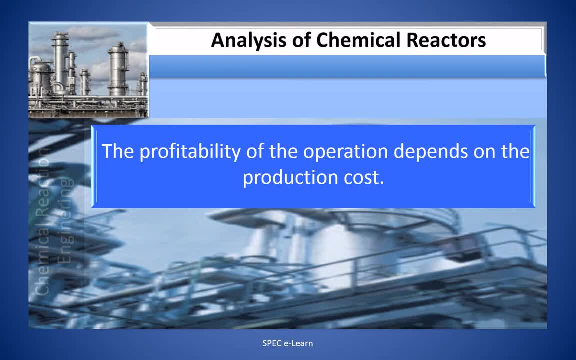 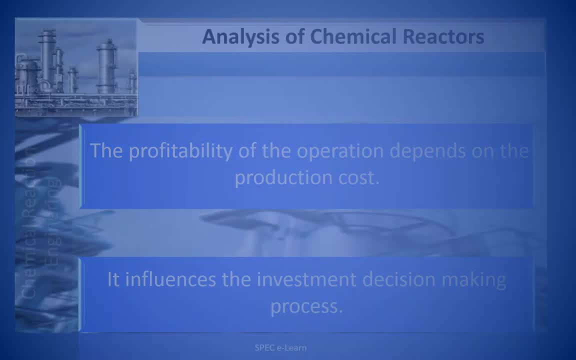 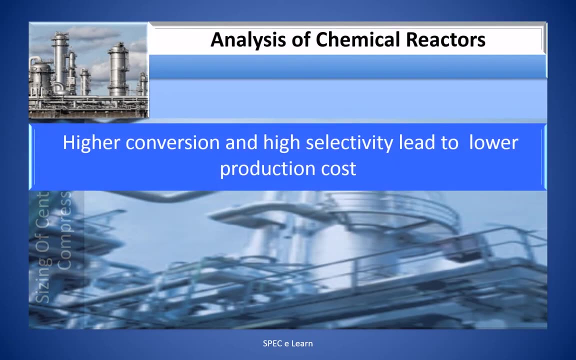 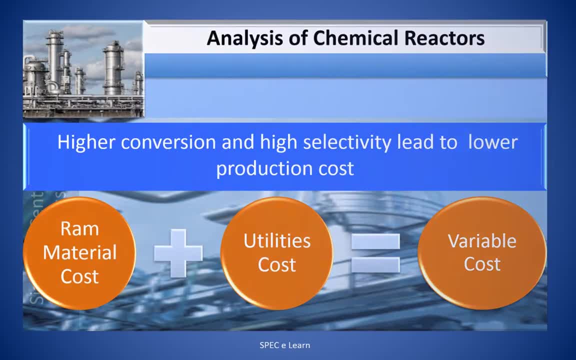 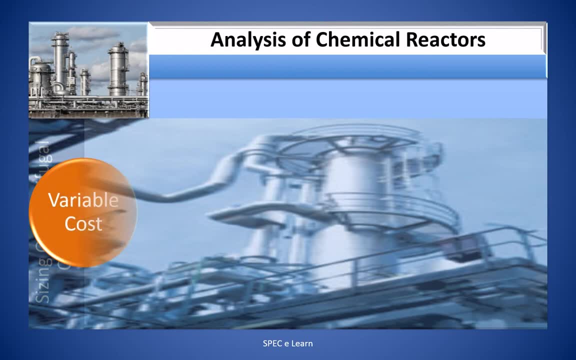 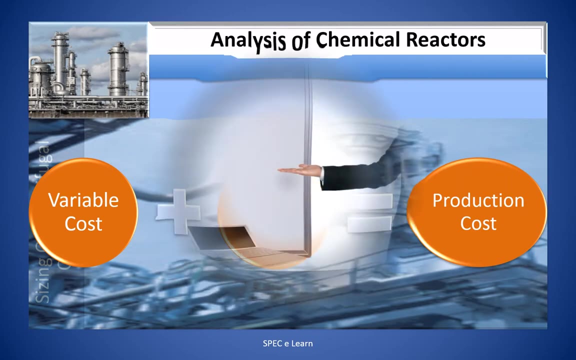 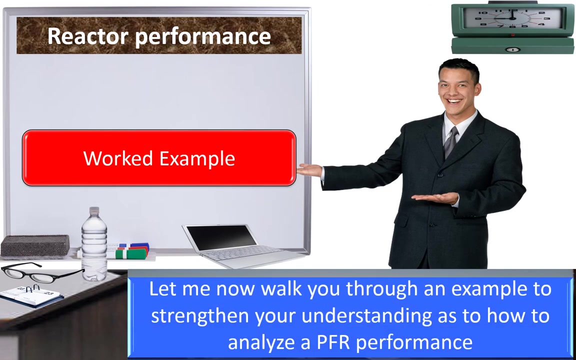 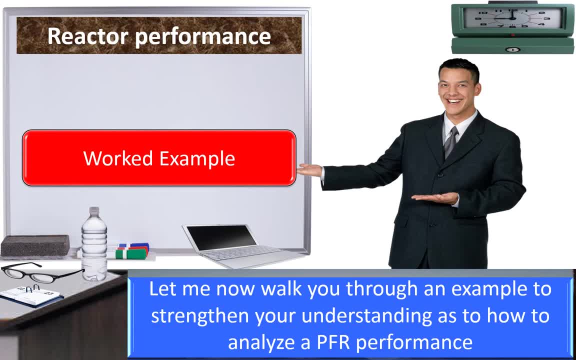 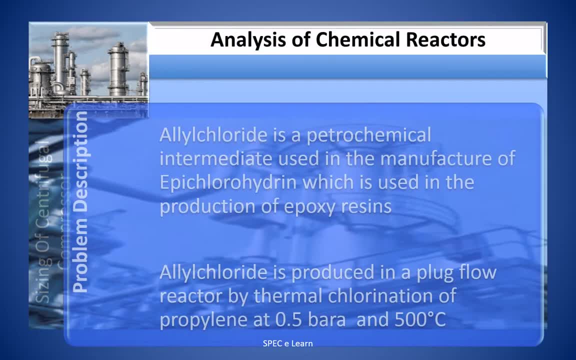 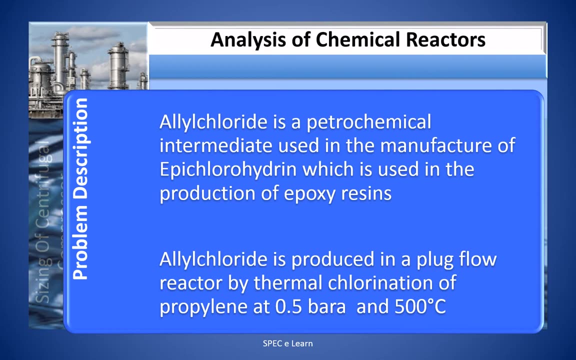 PO4 performance. The problem description. Allyl chloride is a petrochemical intermediate used in the manufacture of apichlorohydrin, which is used in the production of epoxy resins. Allyl chloride is produced in a plug flow reactor by thermal chlorination of propylene. 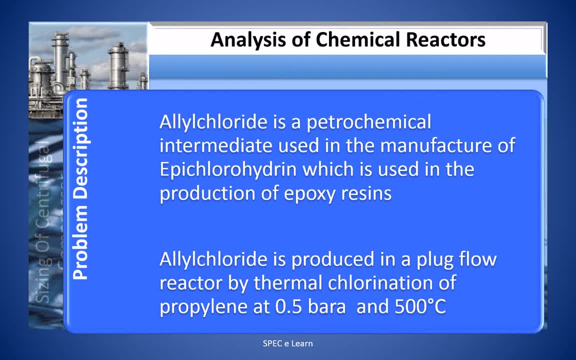 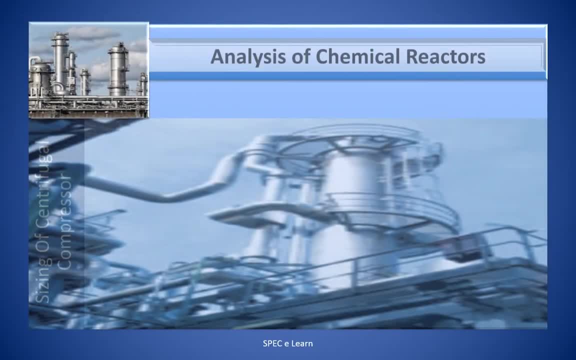 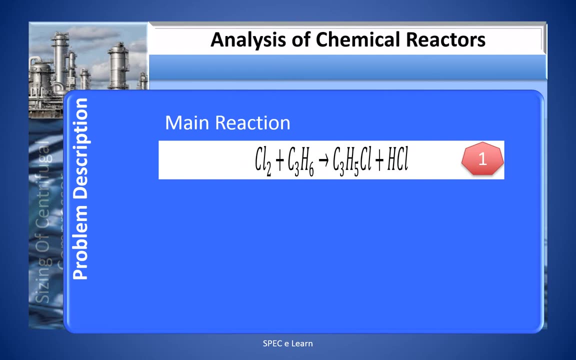 at 0.5 bar absolute pressure and 500 degree centigrade. The key reactions occurring in the reactor at the specified operating conditions are described here. The main reaction is a substitution reaction between propylene and chlorine to form allyl chloride and hydrogen chloride. 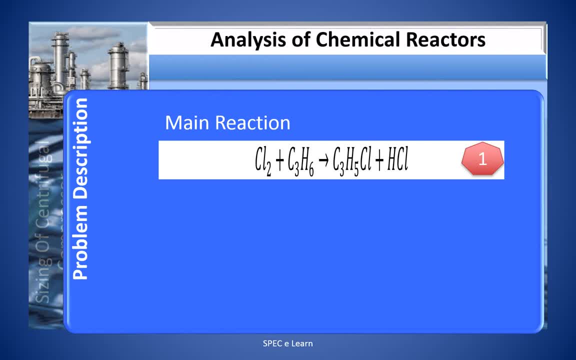 In parallel to the main reaction, side reaction is also taking place which is an addition reaction between propylene and chlorine to form dichloropropane. There are some other series reactions are also occurring which results in consumption of the main product. These are undesired reactions but are unavoidable. 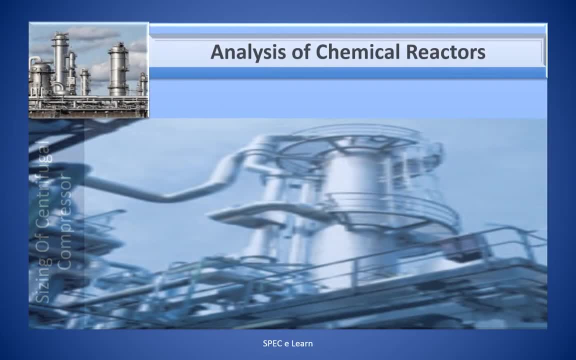 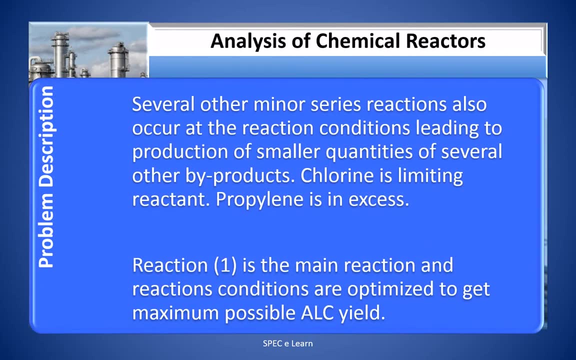 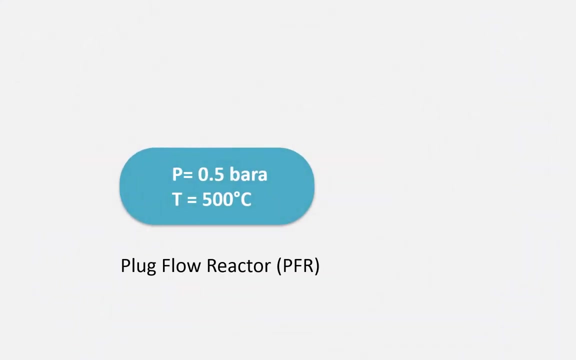 Chlorine is a limiting component and propylene is used in excess. Reaction 1 is the main reaction and reaction conditions are optimized to get the maximum possible allyl chloride yield. This figure illustrates the plug flow reaction. This figure illustrates the plug flow reaction. 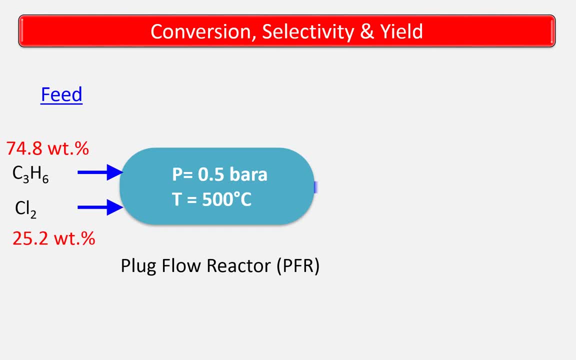 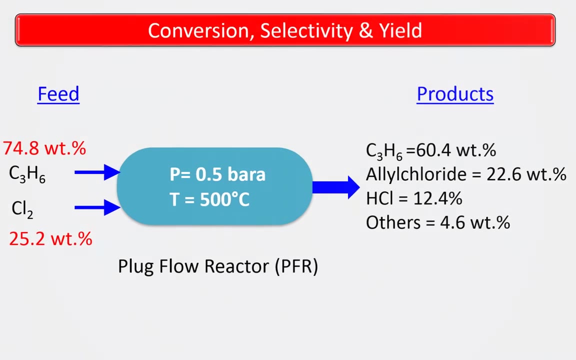 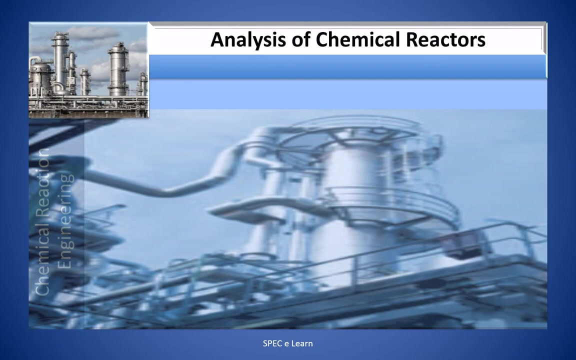 This figure illustrates the plug flow reaction. In another case, allyl chloride is the only content of this reaction at the AKA Oing combined feed ratio for the main rigid reaction. Now let us proceed to see another reaction to solve the 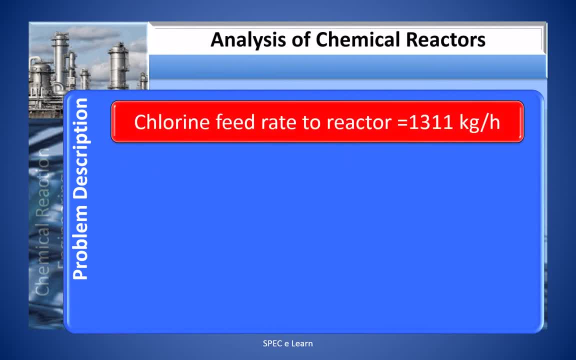 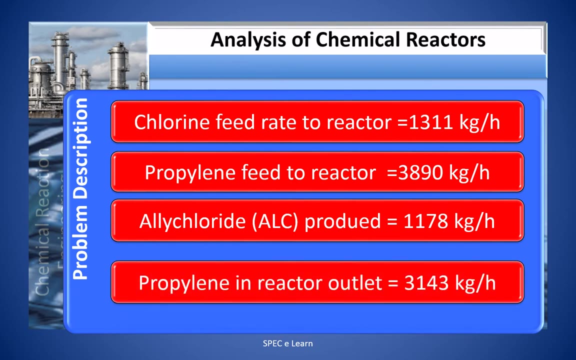 Populin feed rate to the reactor is 1311 kg per hour. Populin feed to the reactor is 3890 kg per hour. Allyl chloride produced is 1178 kg per hour. Populin in reactor outlet is 3143 kg per hour. 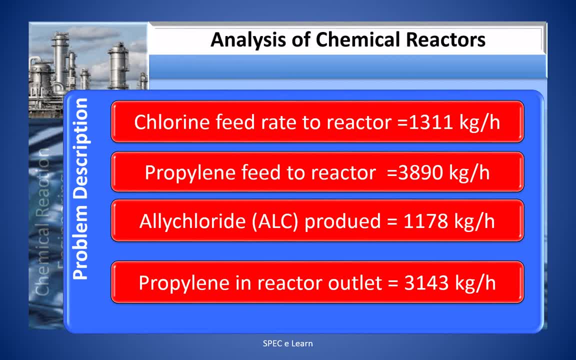 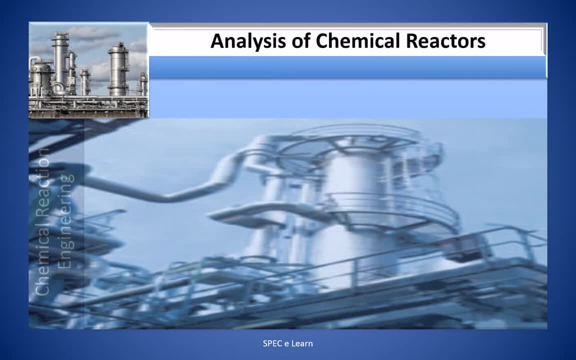 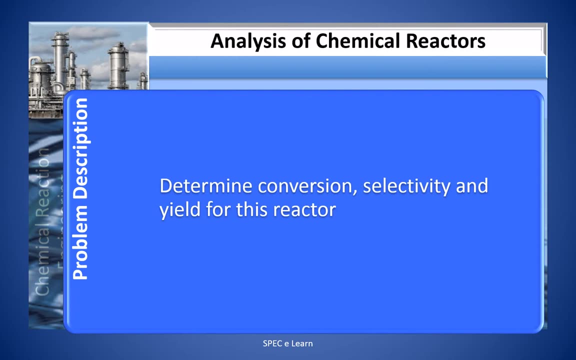 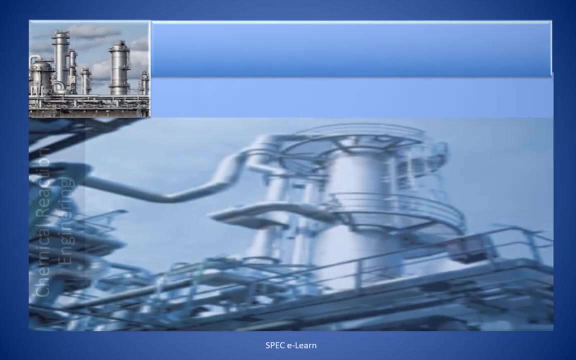 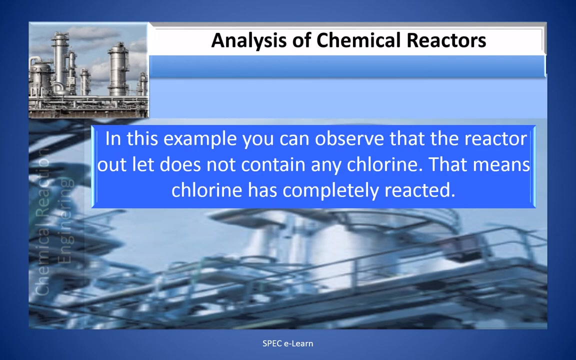 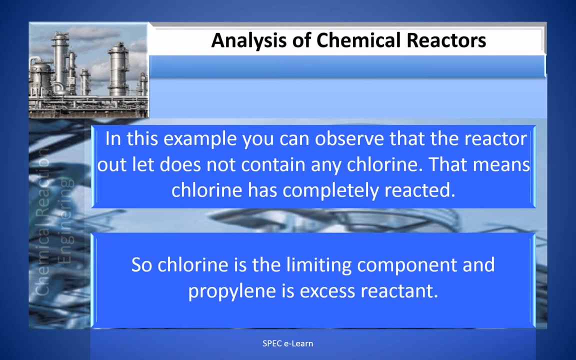 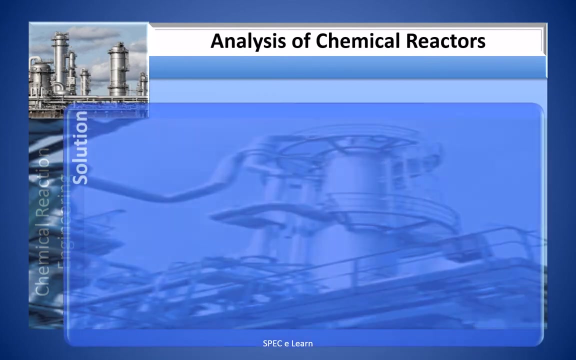 These flows are taken from a real world example. You are required to determine conversion selectivity and yield for this reactor. In this example, you can observe that the reactor outlet does not contain any chlorine. That means chlorine has completely reacted. So chlorine is the limiting component and propylene is the excess component. 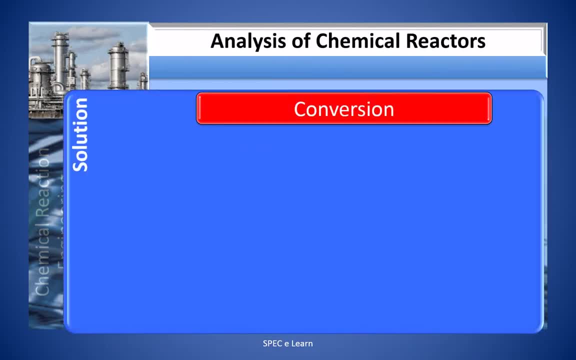 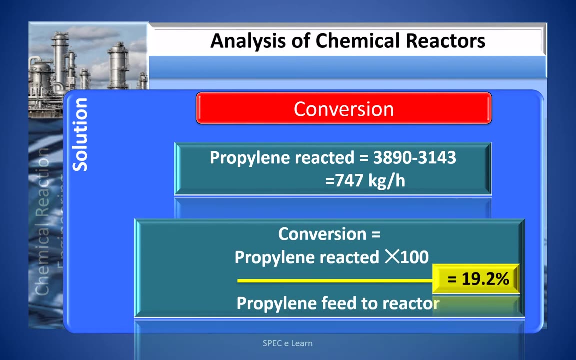 You can use the mass flow rates to determine the conversion and other parameters. You can also use the concentration terms to determine the conversion. To determine the conversion, First determine the populin reactant, which is 747 kg per hour. So the conversion is populin reactant divided by populin feed to the reactor which works. 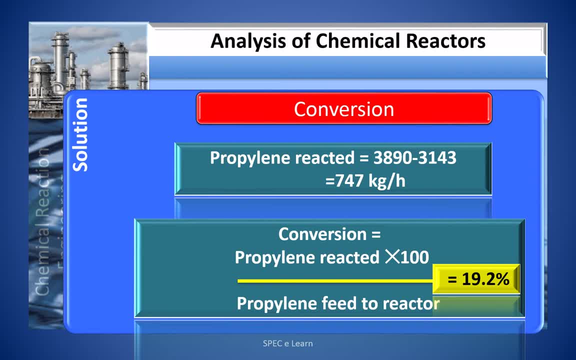 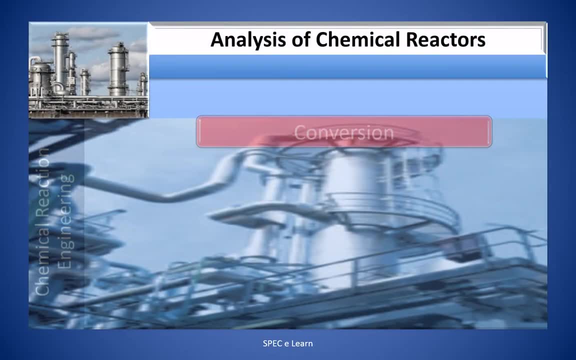 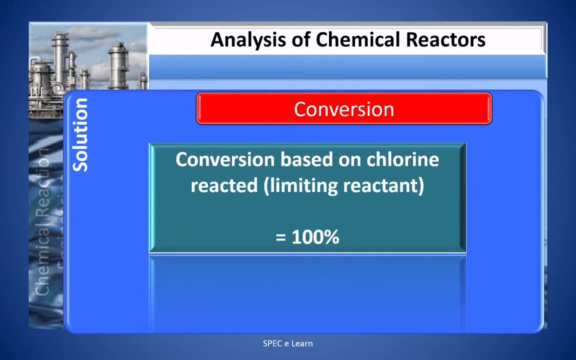 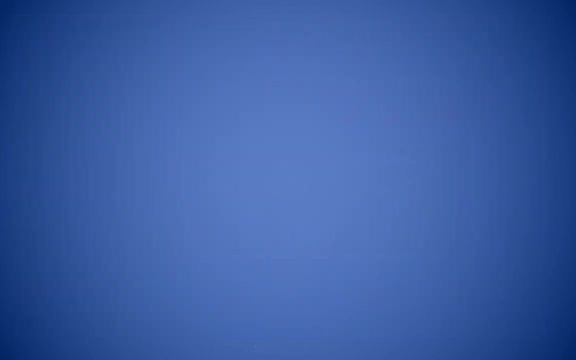 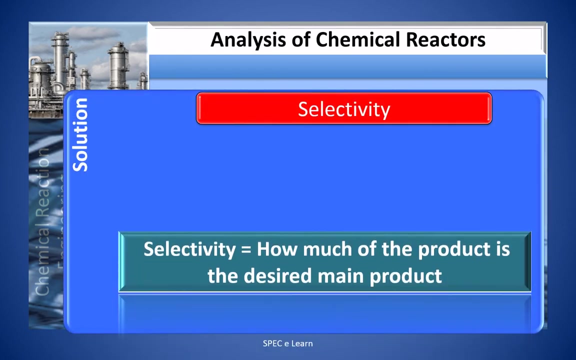 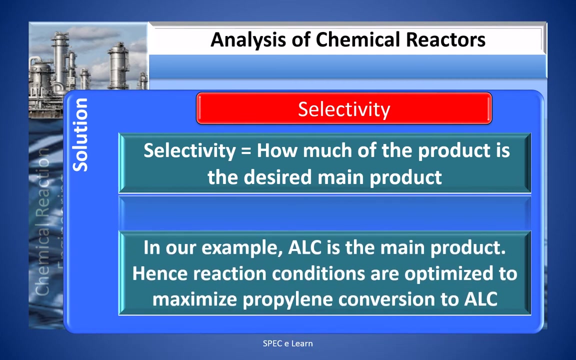 out to 19.2%, As expected. the conversion based on chlorine reacted is 100% because chlorine concentration in the outlet is 0.. Selectivity: Selectivity is how much of the product is a desired main product. In our example, allyl chloride is a main product. 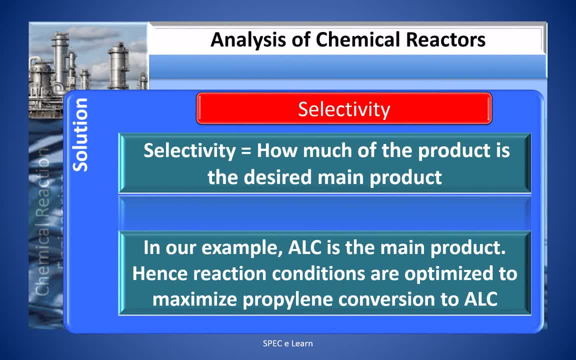 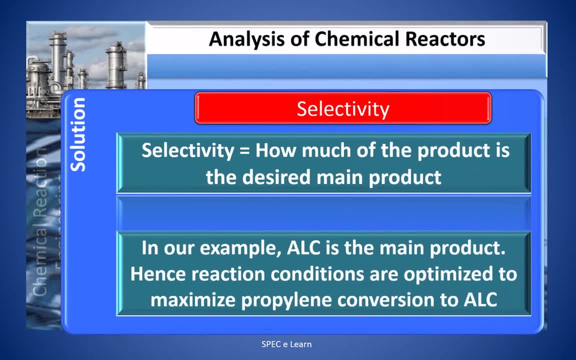 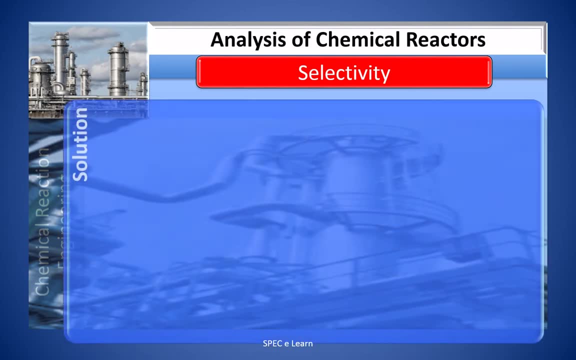 Hence the conversion is 100%. Selectivity is how much of the product is a desired main product. Hence the conversion is 100%. In the next head case, reaction conditions are optimized to maximize propyl conversion to allyl chloride. The concentration of byproducts is 4.6%. 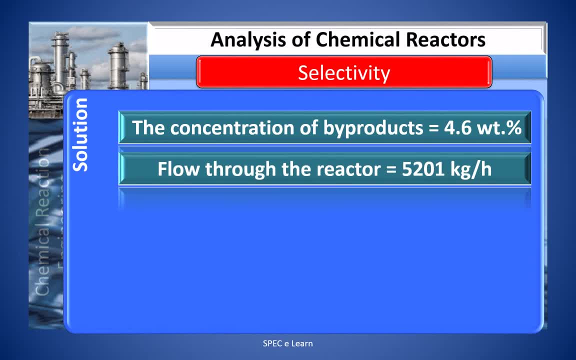 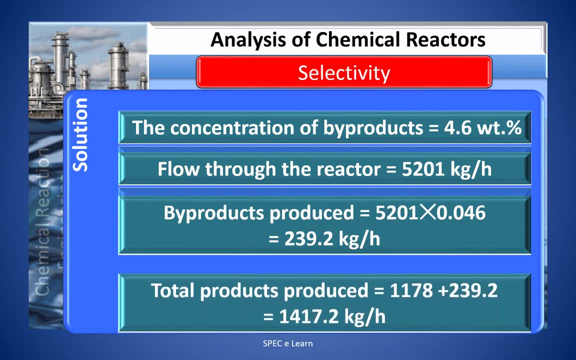 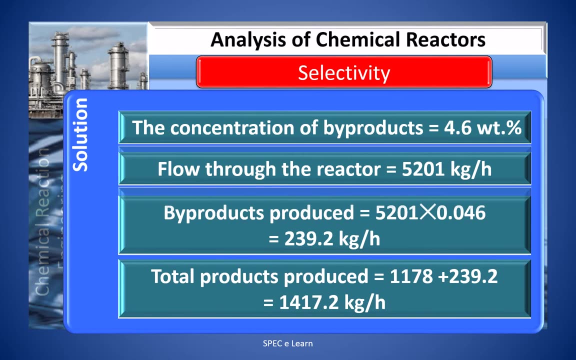 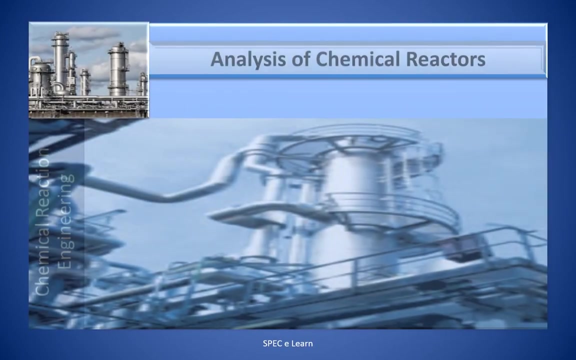 The weight Flow through the reactor is 5,201 kg per hour. Byproducts produced is 239.2 kg per hour. So the total product produced is 3,734 kg per hour. So total product produced is 1417.2 kg per hour. 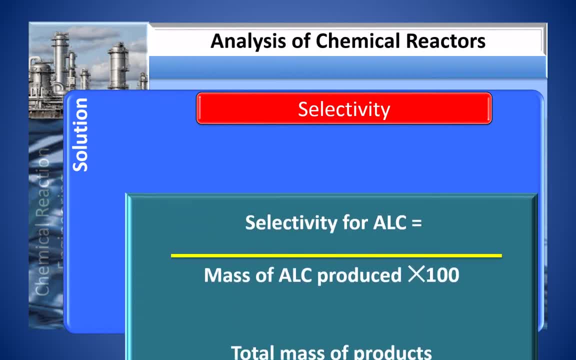 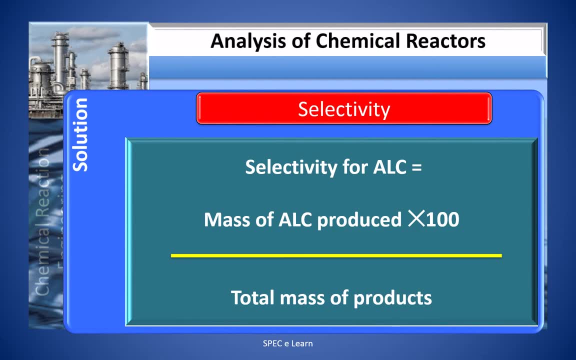 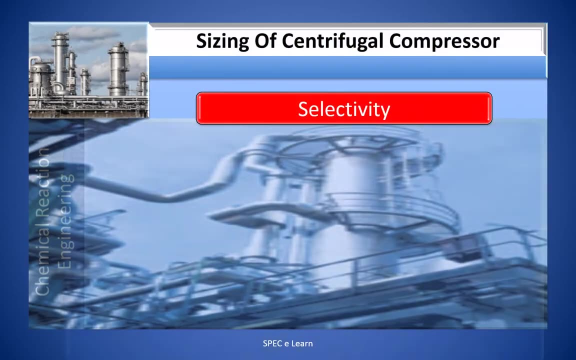 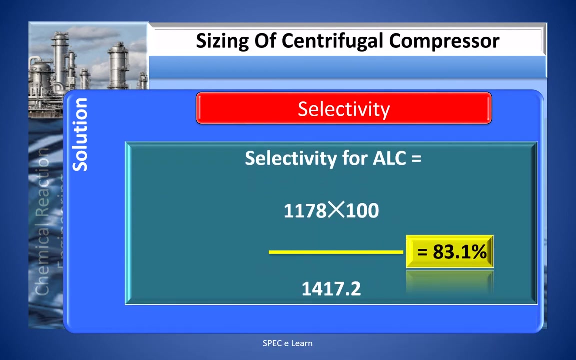 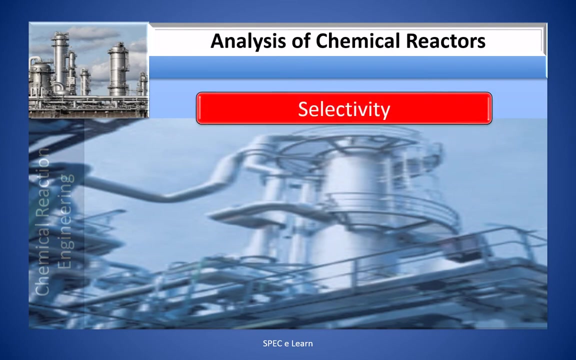 So selectivity for ALC is the mass of ALC produced divided by total mass of products Substituting their values. you get the selectivity of 83.1%. Selectivity: 83.1%. What is the meaning of this? 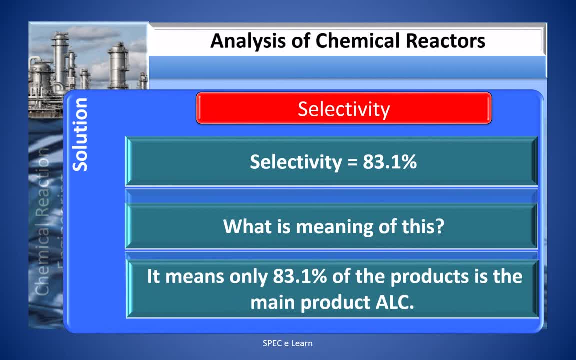 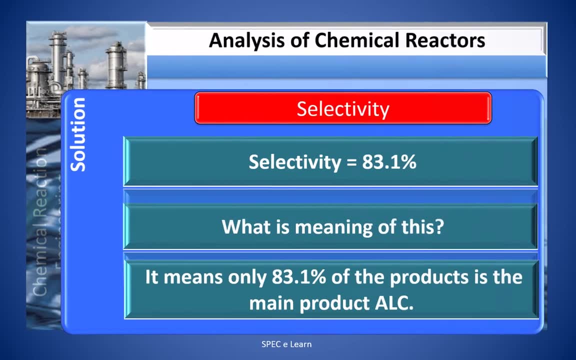 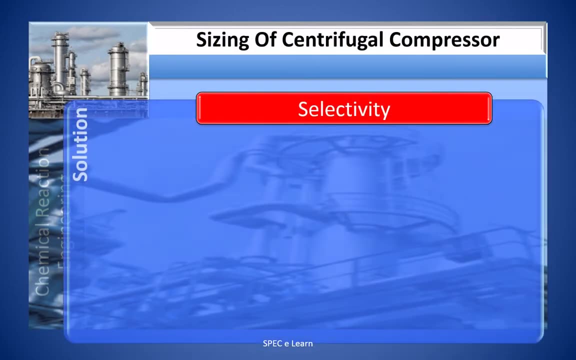 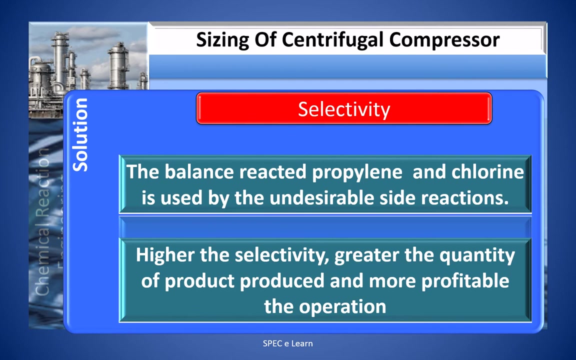 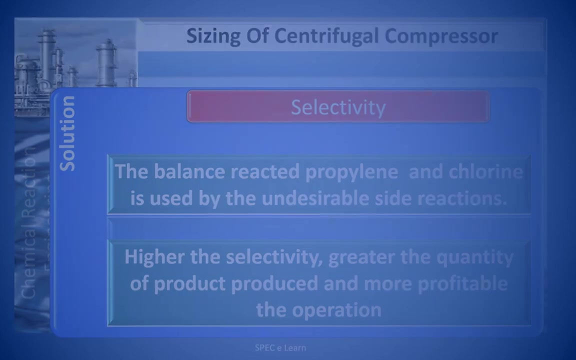 It means only 83.1% of the products is a main product. ALC. The balance reactant, propylene and chlorine, is used by the undesirable side reactions. Higher the selectivity, greater the quantity of product produced and more profitable the operation. 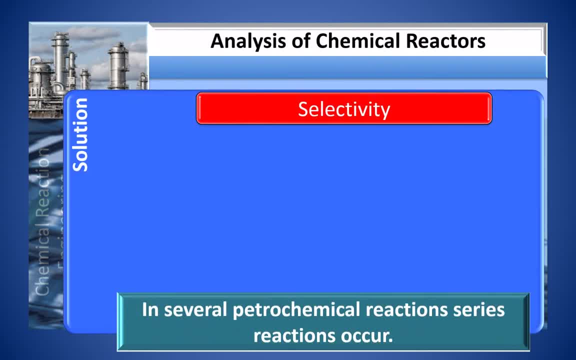 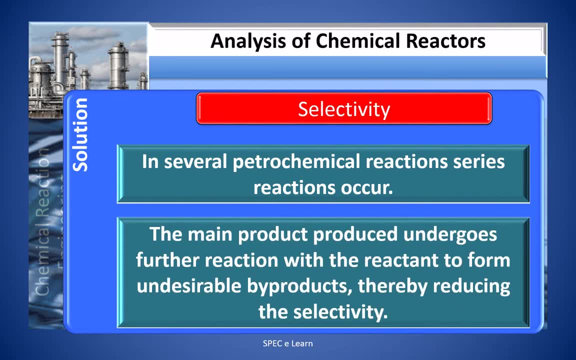 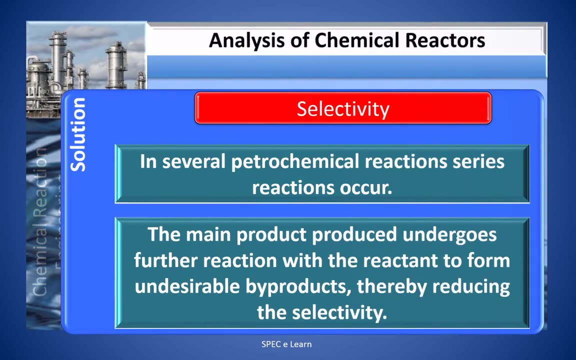 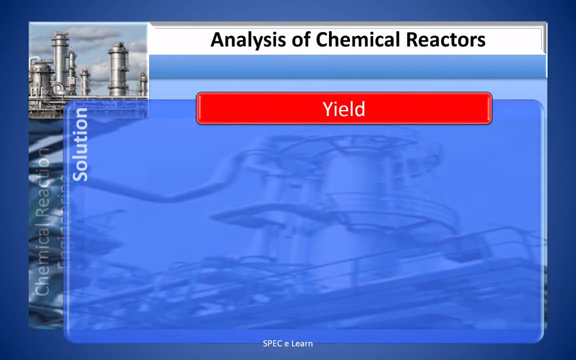 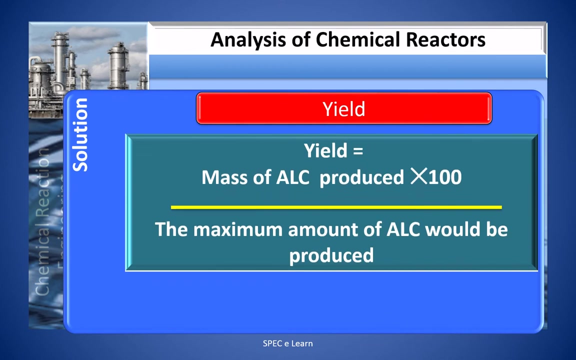 In several petrochemical reactions series, reactions occur. The main product produced undergoes further reaction with the reactant to form undesirable byproducts, thereby reducing the selectivity. What is yield? Yield is the ratio of mass of ALC produced to the maximum amount of ALC would be produced if there were no side reactions. 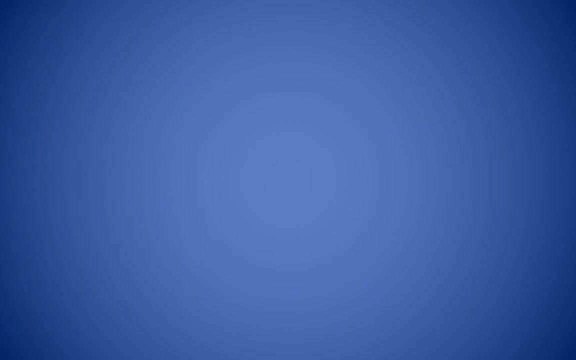 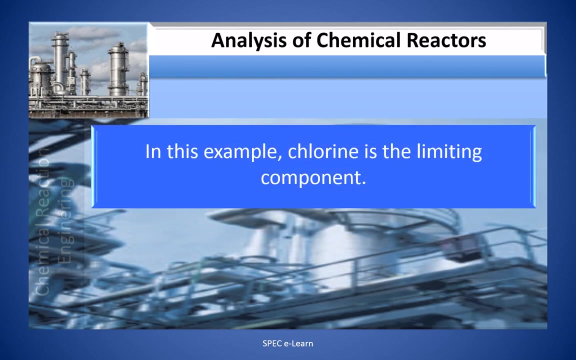 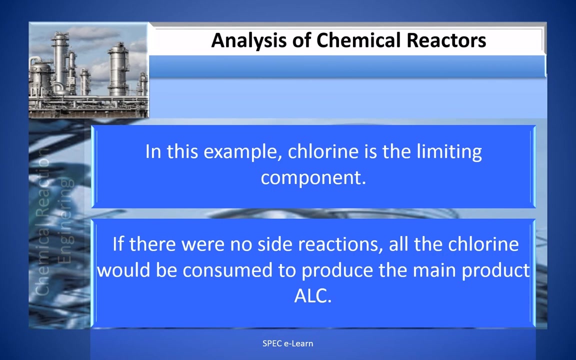 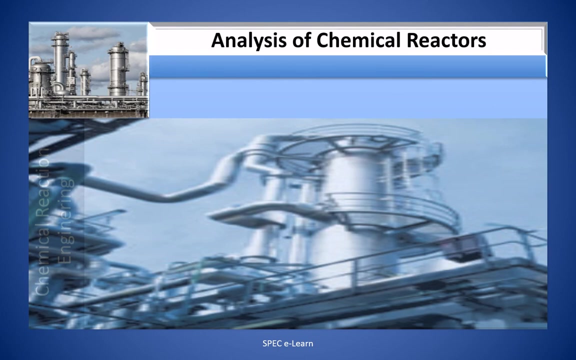 What is chlorine? In this example, Chlorine is the limiting component. If there were no side reactions, all the chlorine would be consumed to produce the main product, ALC. So the maximum possible amount of ALC possible to produce is 1412 kg per hour. 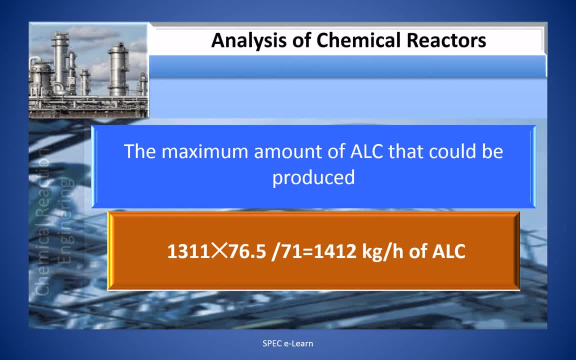 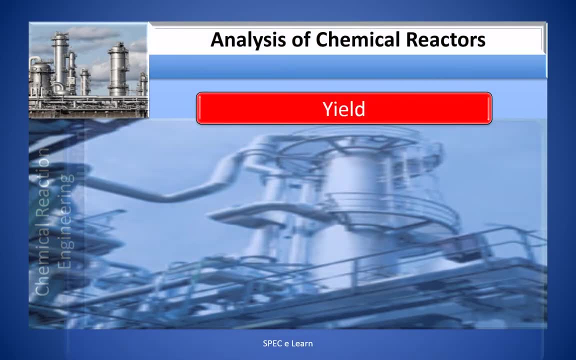 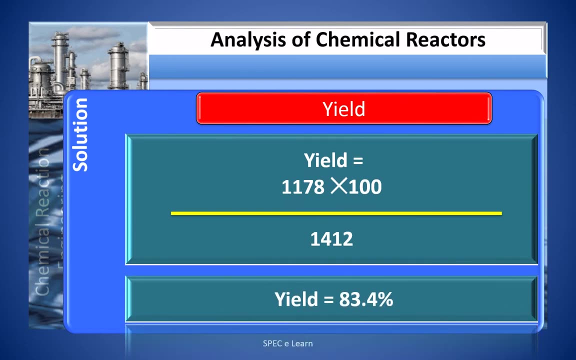 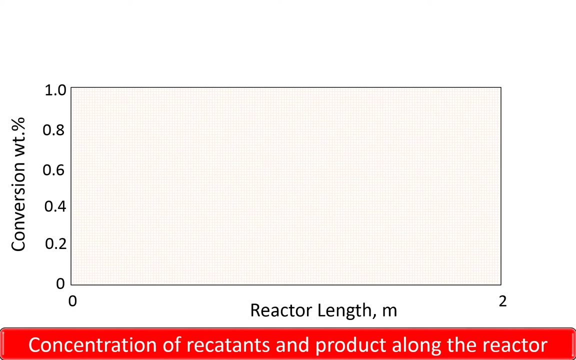 So the yield is 83.4%. So the yield is 83.4%. This graph is an illustration of the change of concentration of reactants and products along the legion. Chlorine being the limiting component, decreases progressively and becomes zero at the end of the reactant.